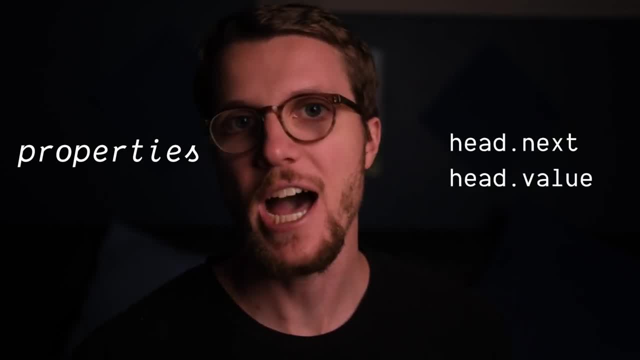 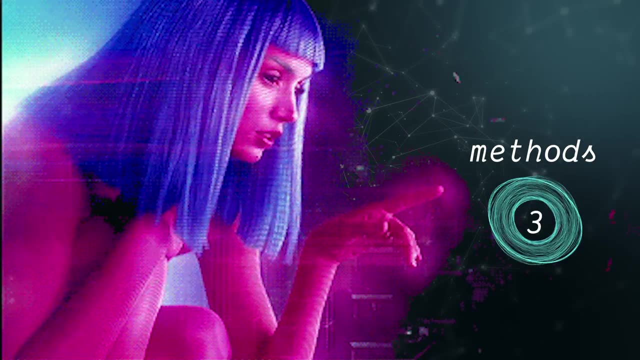 We already talked about two properties: dot next and dot value. They just give us info that's stored on our node. Methods, on the other hand, can perform actions on the node, changing this info or doing different things to our list. In other words, they're functions. 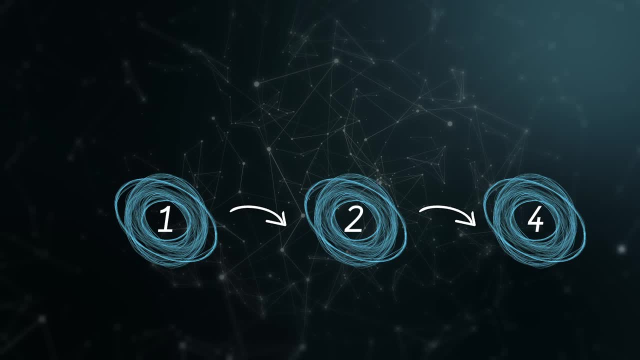 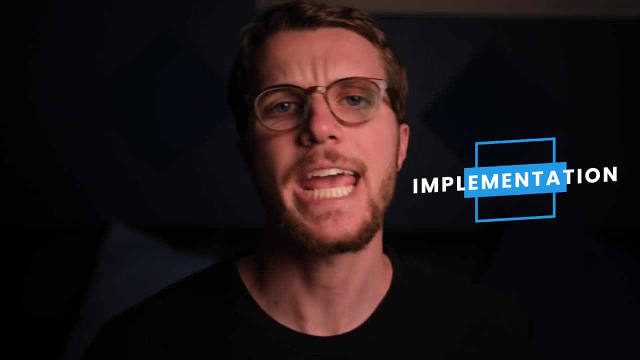 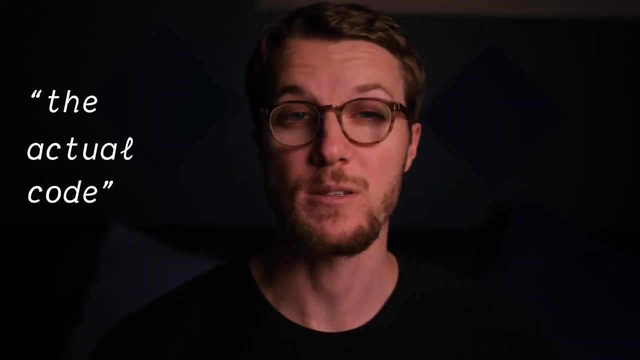 stored on an object. An example of a method would be adding a new node to the end of the list or retrieving the value it indexed. Now, what's implementation? It's how we actually code our data structures and our methods. You can write the same method a hundred different ways, with terrible spaghetti code. 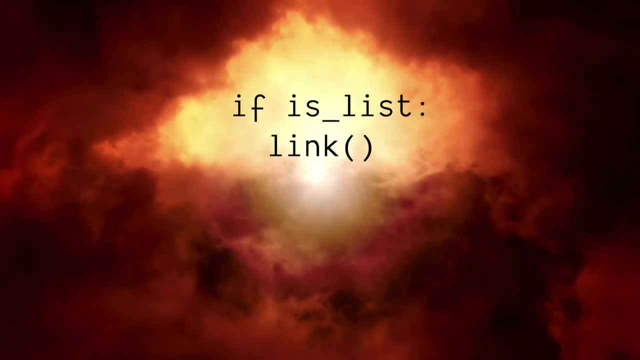 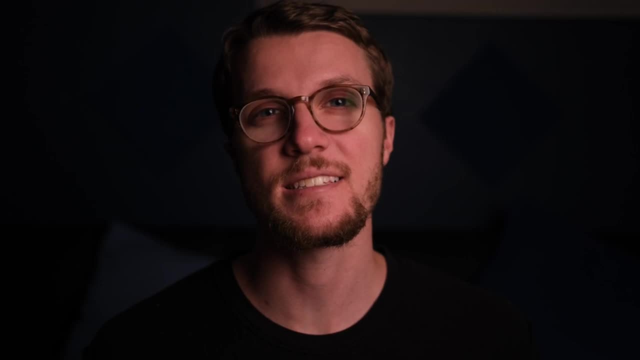 that's really slow or the most beautiful code you've beheld in your life, And luckily you can't finish too fast in programming. The important thing is that they work, though The interface doesn't care how methods are coded under the hood, Just like someone who's. 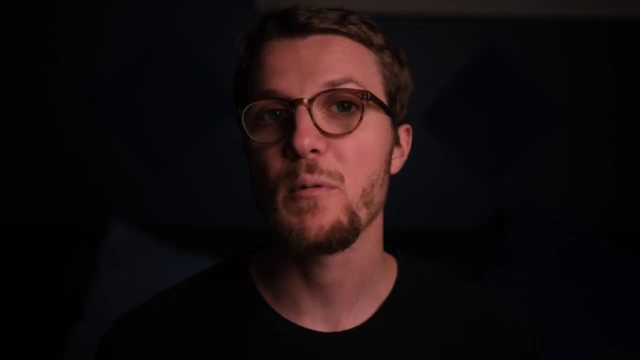 viewing your website, doesn't care how that code looks. In any case, that's it for this video. Thanks for watching and I'll see you in the next video. In this case, now we can talk about the implementation and interfaces of a linked list. 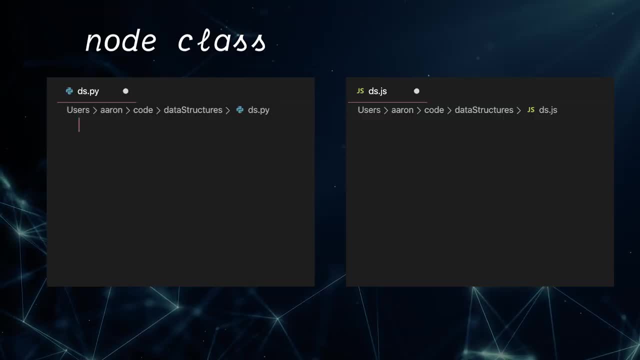 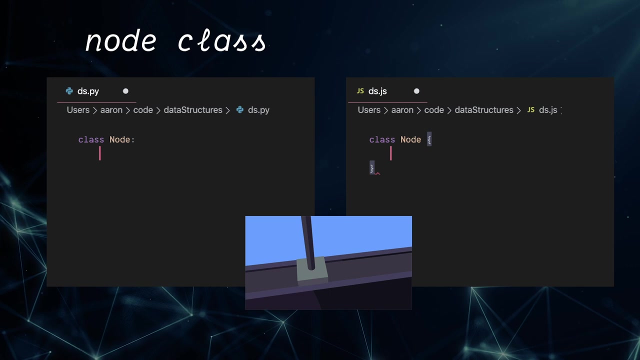 Let's implement a node as a class. You have classes in every language that supports object-oriented programming. JavaScript and Python are the two I like most, But classes always have a few things in common. Think of a class as a factory that creates objects. So with one. 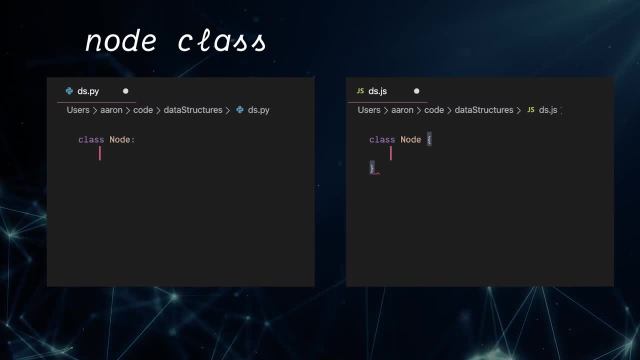 node class. I can create as many nodes as I want. Classes always have an init or constructor function which tells the class how to set things up. There also needs to be a way for the object to reference itself, which we'll use the self or the this keyword to do To tie this all together, if we want to create 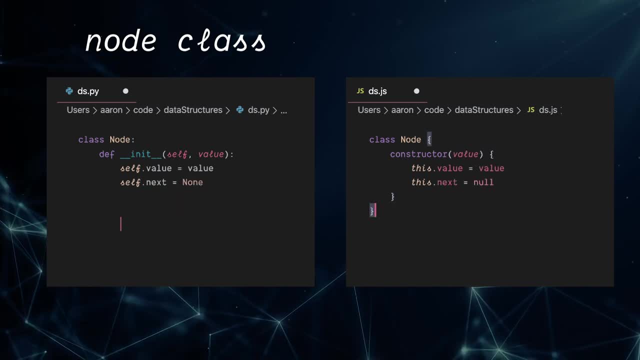 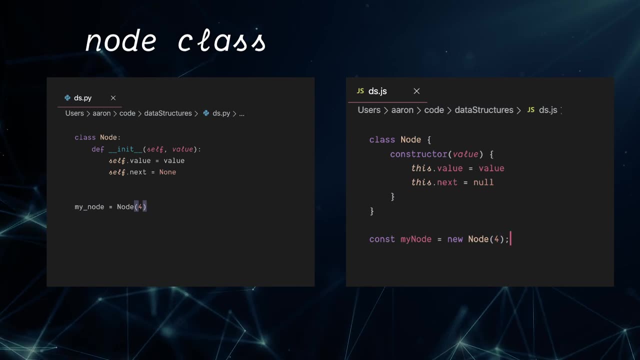 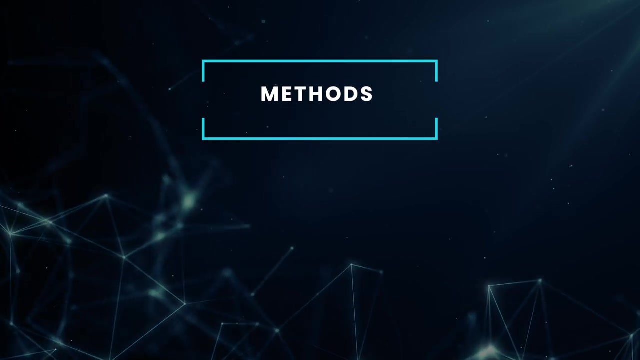 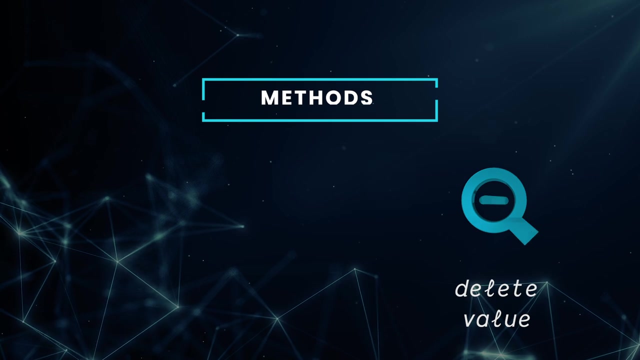 a node with value 4, we have to set selfvalue to 4.. We'll also set next to none, meaning this is the tail of a list. Let's think of methods we'll definitely need in our interface to do different things to our list, Namely addToTail: get from an index in our list and to delete a value from. 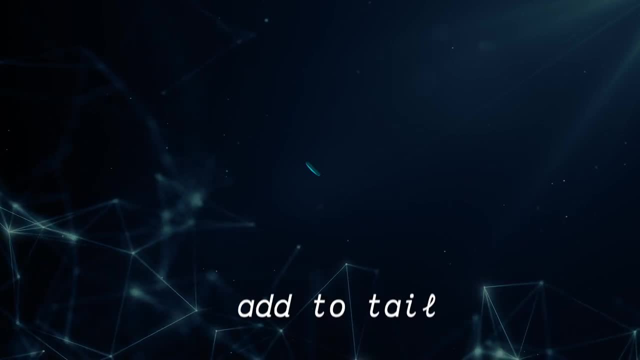 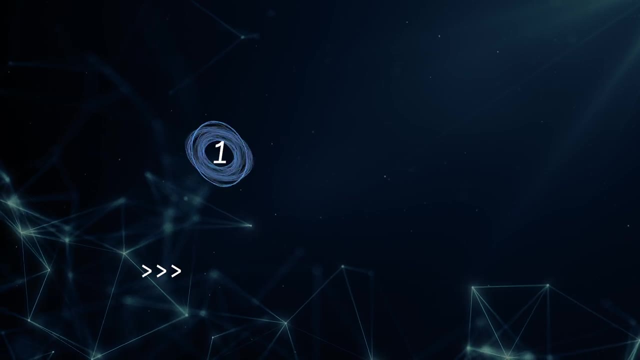 the list. Let's start off with the addToTail method. We'll initialize our list with a new node. This part's really important. We can move throughout our list by storing a pointer to the variable on keeping track of our current position. 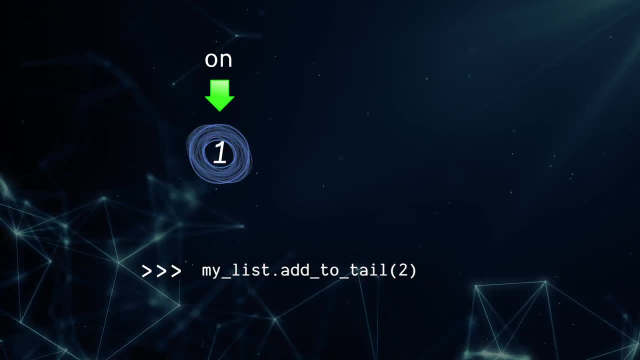 Here we want to move on for the list. We can also store a pointer to the variable on keeping track of our current position. Here we want to move on for the list. Here we want to move forward until we find the end of our list. 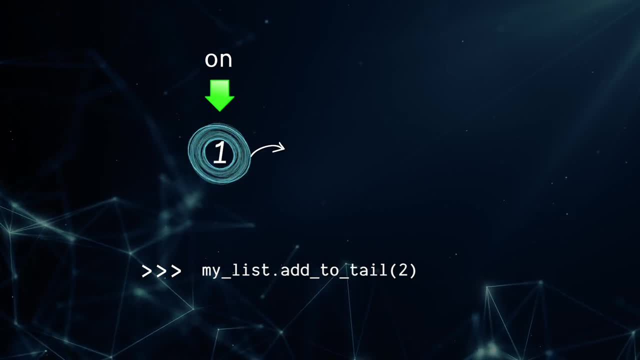 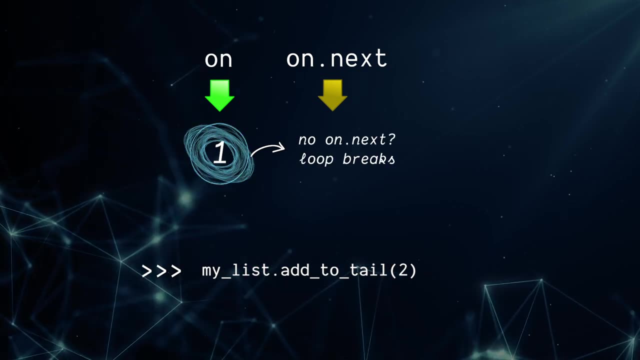 18, We'll create our arms with each example typing at different times. We do this by setting on to on dot next, until we find the end of the list or null. When we hit null, we'll know to create a new node with the value that was passed in. 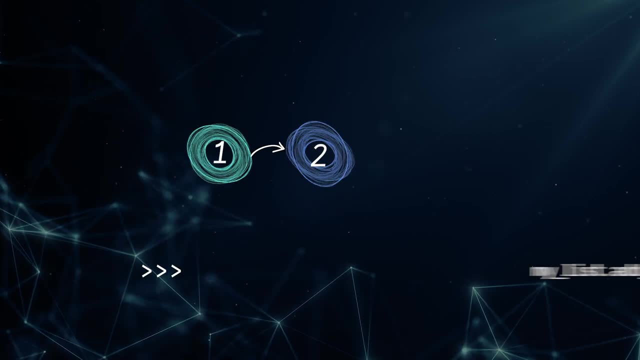 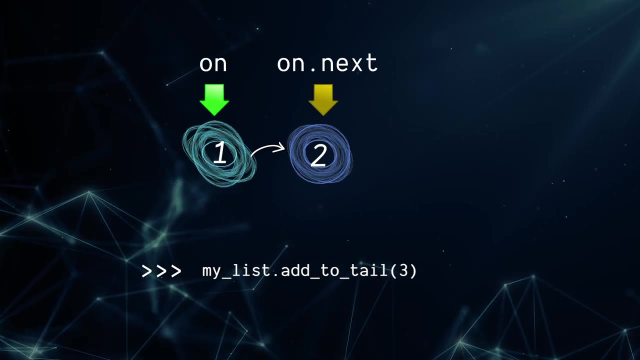 with: Finally, we'll set on dot next to that new node. In this example, where the list is already size 2, you can see on moving forward and then the imply to on dot next moving with it. Finally, when we hit null, we'll add: 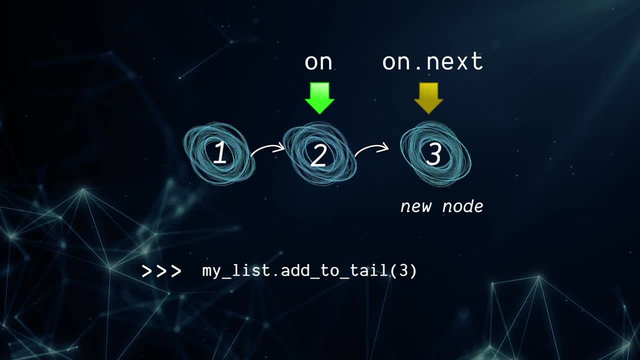 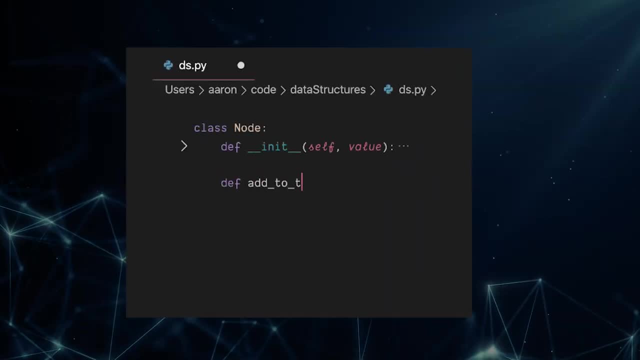 a new third node with value 3. 3.. Finally, let's write some code. I'm just going to write Python code, since the JavaScript is pretty much the same. Let's create that add to tail method on our node class. We'll, of course, 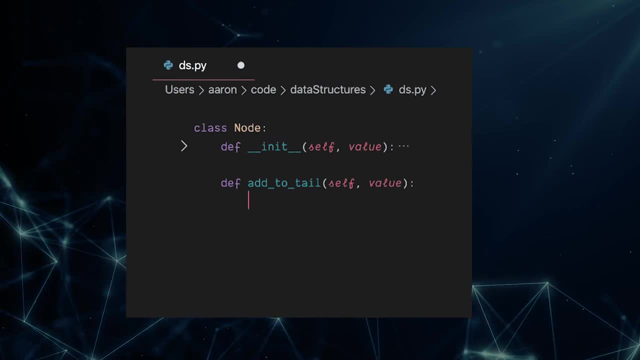 need value as an argument. Remember, in almost all these methods, we're going to need the on pointer to traverse our list, so let's write that first. Since we're writing a loop, we have to think of our break condition, which will be when we hit the end of our list, or onnext is none. 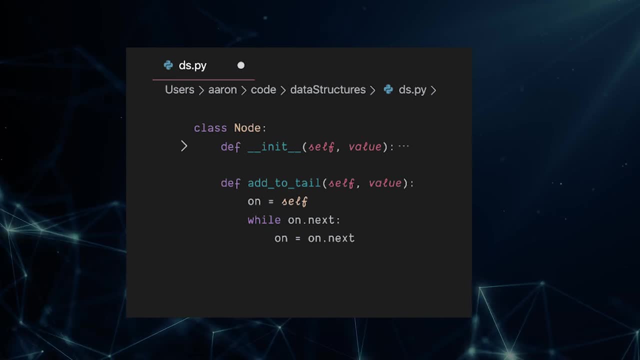 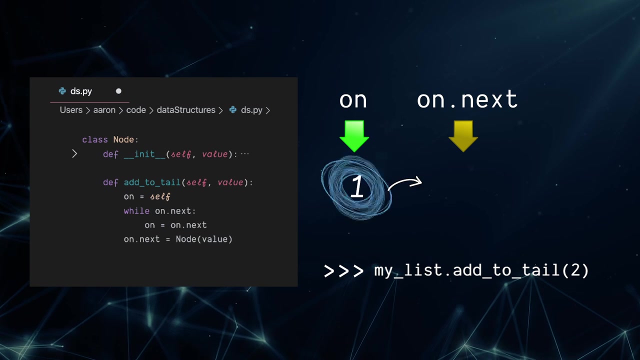 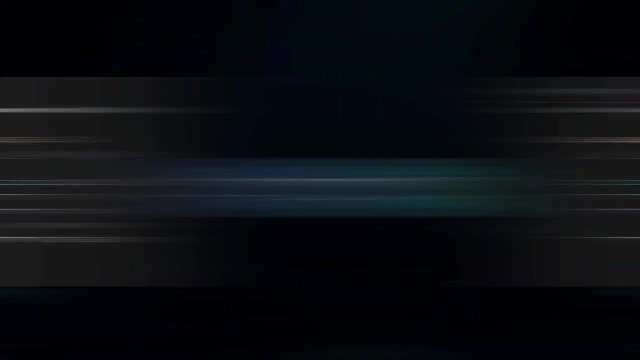 Finally, in the body of the loop, we'll advance on forward. Then, after our loop breaks, we'll set onnext to a new node, that is, the node being added to the tail. We've written our code, so let's see the add to tail method in action. You probably noticed that every time we run this 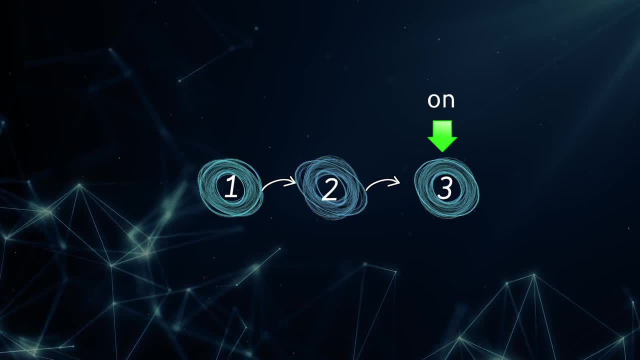 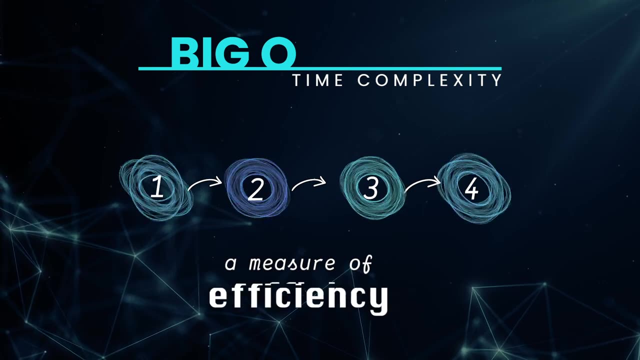 we have to touch every node in our list before adding a new one to the end. That's where the big O, or time complexity, comes in. It's a measure of the efficiency of our add to tail method. Let's just pretend that each time our loop runs. 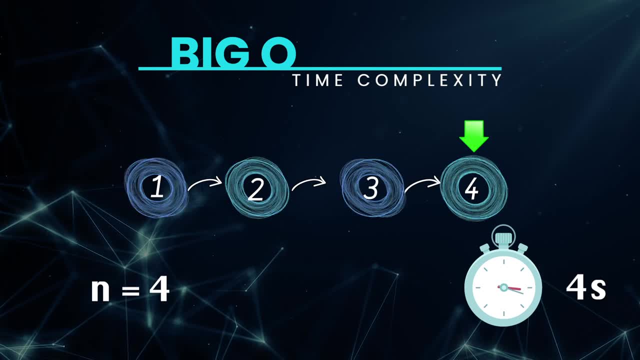 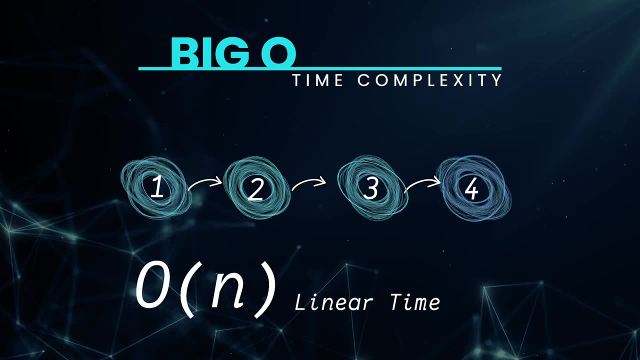 it takes a full second. If n is the number of nodes in our list, add to tail will take n seconds to complete. This makes our time complexity O of n, or equal to the number of nodes in our list. In technical terms, it scales linearly with our input Moving on. let's retrieve a value. 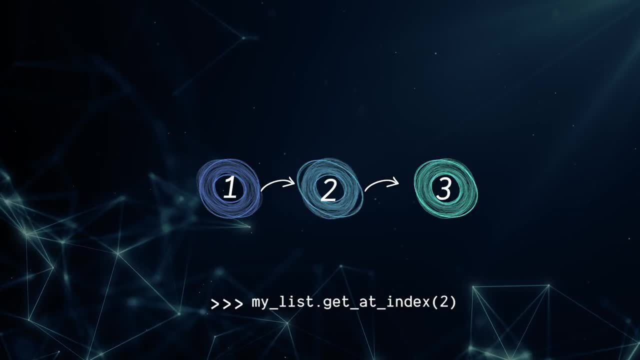 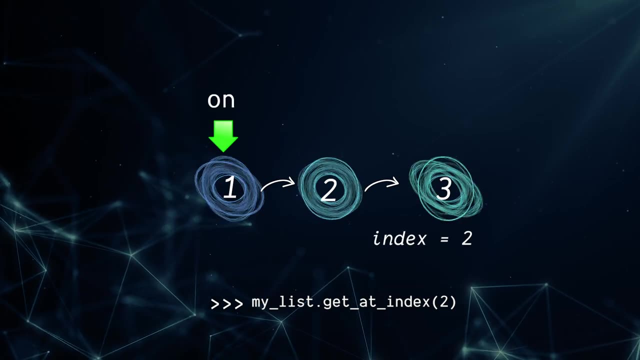 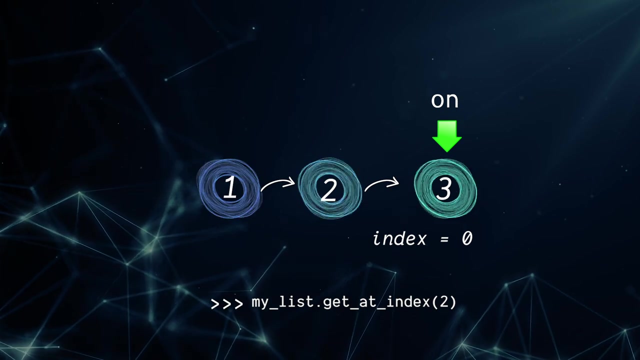 using an index, We'll start with a pre-built list, Unlike an array, we can't use direct indexing to retrieve a node By using the same on pointer method again and decrementing our index every time we advance. we can count down until finding the node we want. Once that happens, we just return the value. 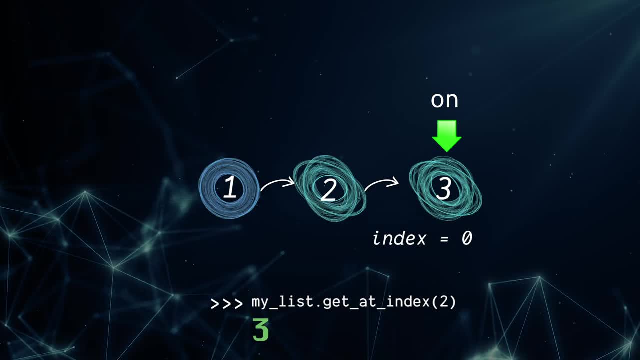 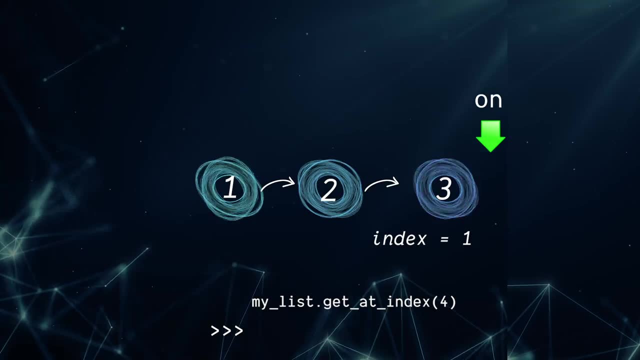 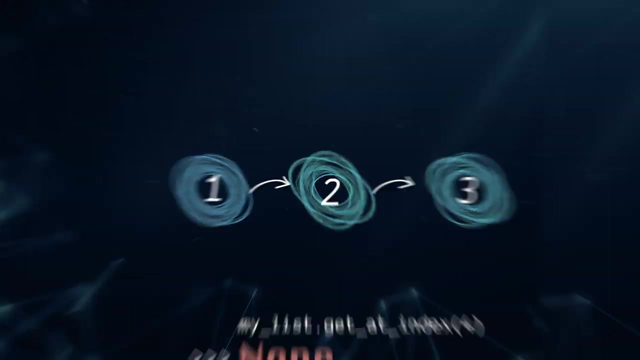 of that node With this method. we do have an edge case, though, Namely what if we try to get an index that is out of the range of our list? We'll go effectively off the end and have to return some value like none or false. Our method will take the target index as the argument. 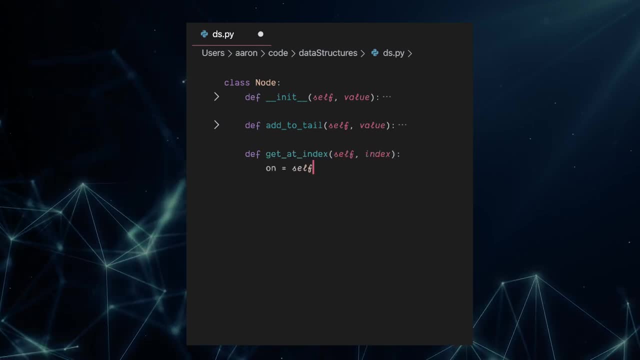 Then our while loop will have to check for either the end of the list or index reaching zero, our terminal conditions Within the loop. we of course are going to want to advance or on and decrement the index, as we talked about, Depending on the final outcome of the loop. 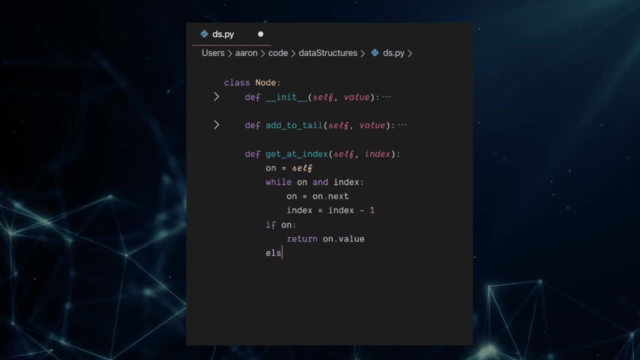 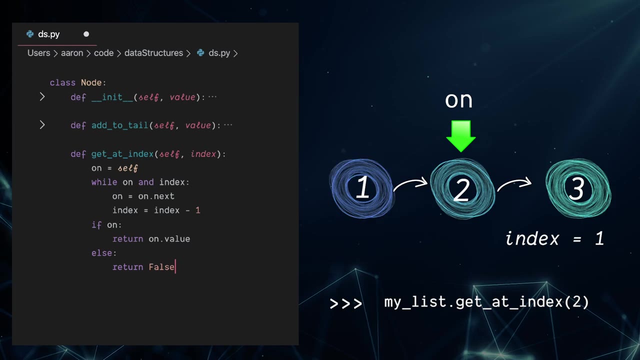 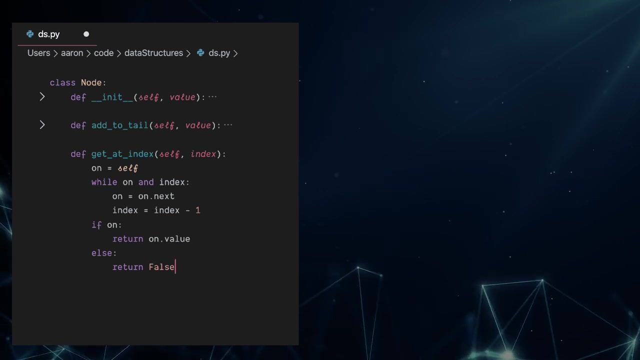 we're then going to use an if statement to either return the value or false. Now let's watch this in action next. Okay, what's our big O this time? With big O, we're pessimistic, meaning we assume the worst case. 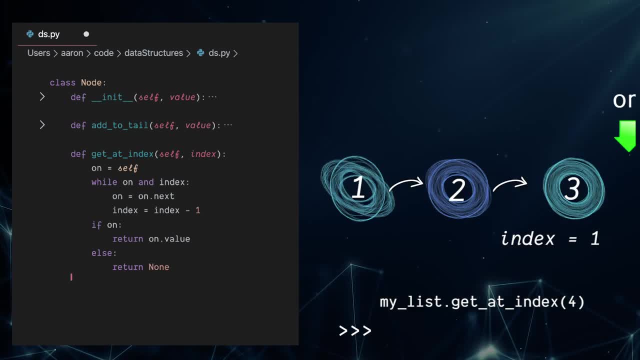 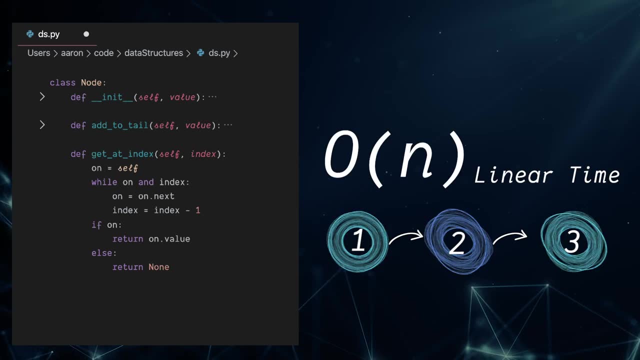 Here the worst case is, of course, falling off the end of our list. When that happens, we traverse the whole list without finding our index, Like last time, when we touch each node exactly once we're running an O of X. So we're going to have to reverse the whole list without finding our index, Like last time, when we touch each node exactly once we're running an O of X. 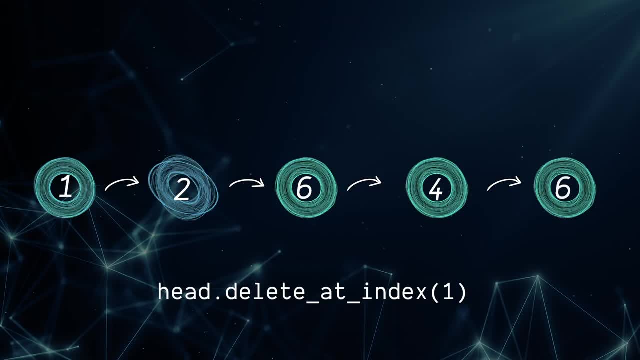 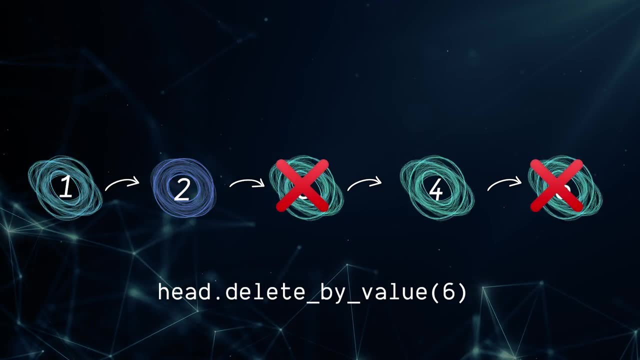 There's a couple different ways we can implement delete. First, we could delete, add an index. On the other hand, we could delete all nodes that match a specific value. Let's assume we do want to delete by value and there could be multiple of the same value. 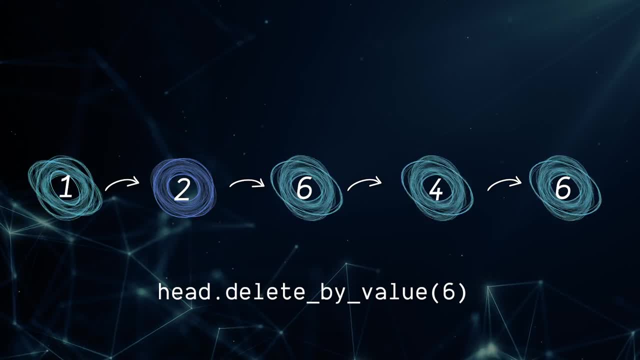 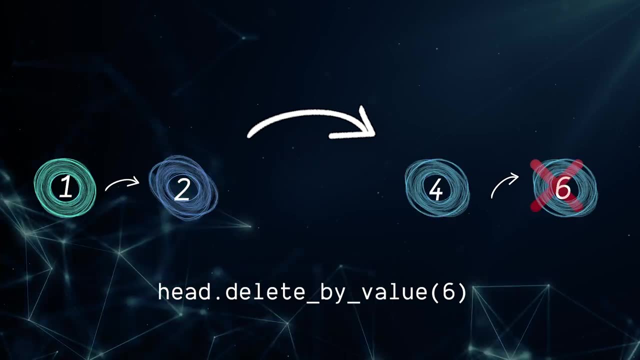 We can infer that by pointing around a node, it's no longer connected to our list. In effect, this deletes our node because there's no more reference to it. If we want to delete the last node, we simply set the second to last to null. 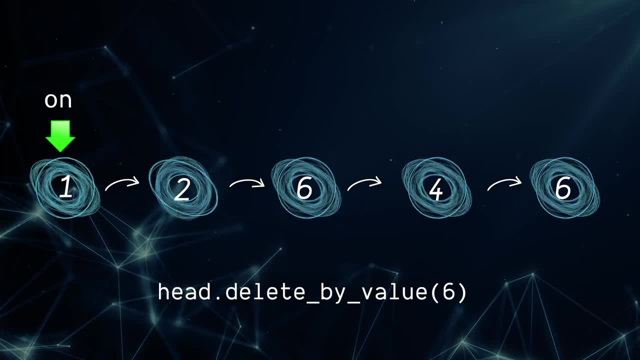 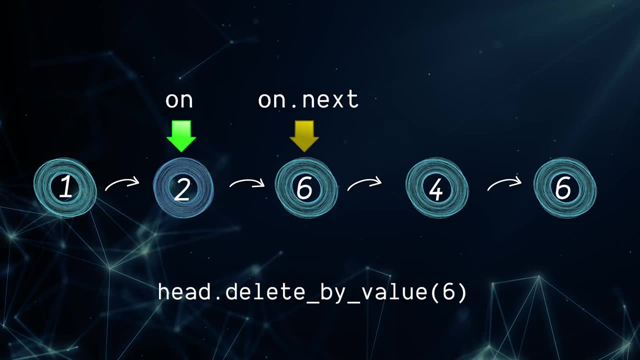 We'll set up our on pointer like normal, except this time we'll have to look to onnext to see if it's a candidate for a deletion. If that's the case, then we'll change our pointer in on to onnextnext or toahead. 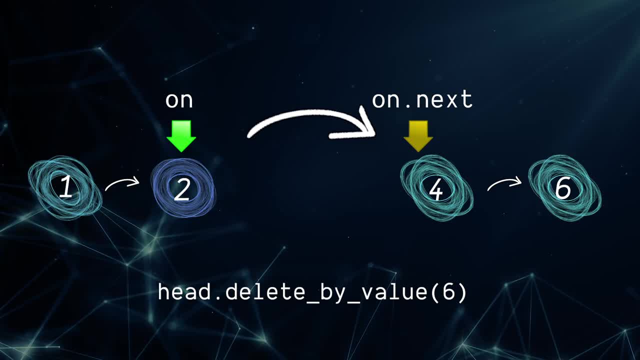 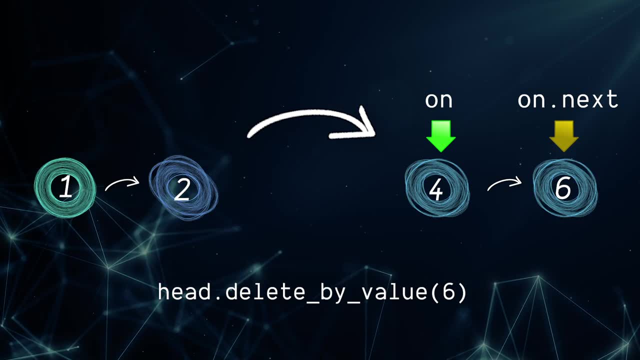 In other words, we set onnext to onnextnext. It's like that node never existed. Now we just move forward our on pointer and continue as normal. When deleting the last node, we have to be careful not to delete it. 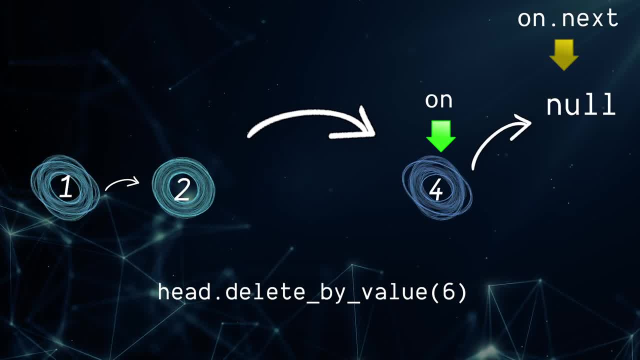 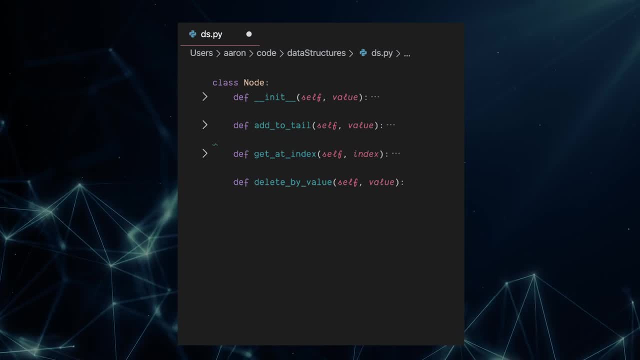 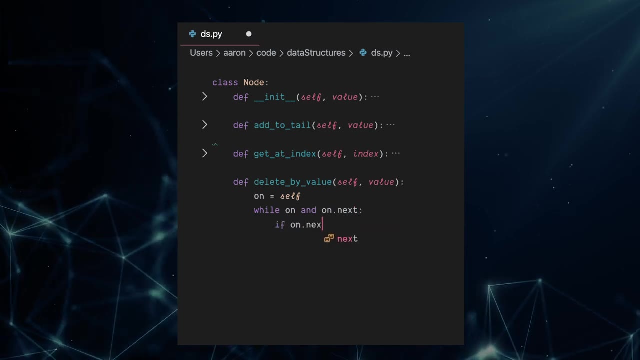 not to go off the end on accident. here's our code. we take, of course, the value slated for deletion as an argument. we set our on pointer, just as we always do, and in the loop we check both on and on. dot next to make sure we don't go off the end accidentally. in the loop we look one. 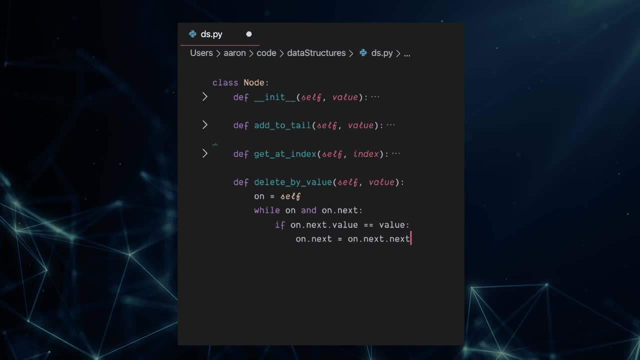 ahead to see if we can delete that value. if so, we set on dot next to on dot, next dot next to point around that node. finally, we advance our on pointer, and that's it, we're done. let's see this one run side by side with the code. 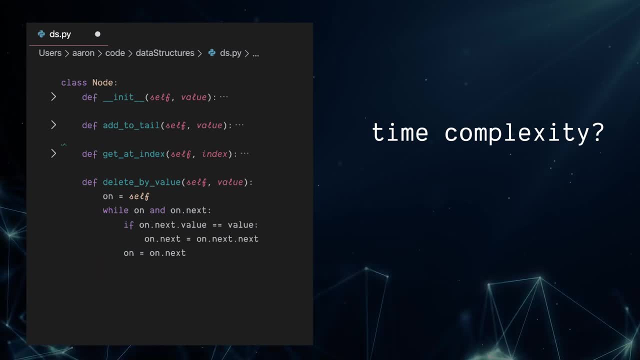 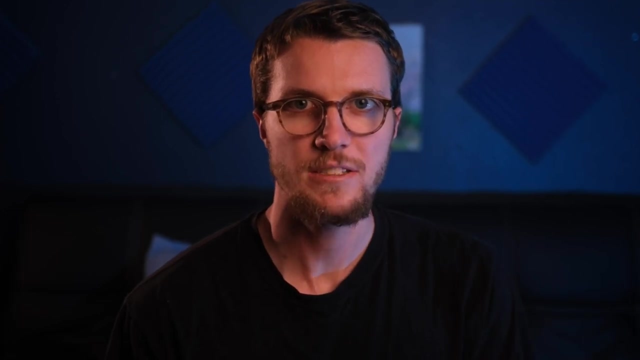 and the time complexity for this one. well, it's pretty straightforward. we're gonna have to check each node at least once to make sure we see all the values. that means linear time, best and worst case. all right, guys, you now know all about linked lists and their common methods. that should give you a really good start for solving linked list. 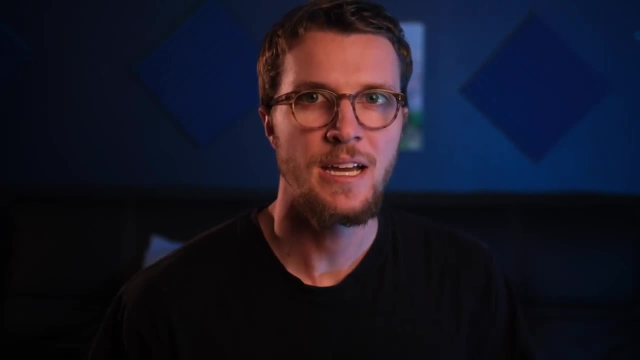 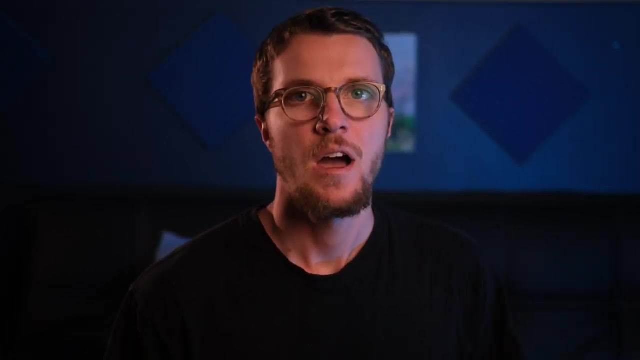 algorithms. if this video gets enough likes, i'll be motivated to do a linked list algorithms video as well. so definitely let me know if you want that. otherwise, i'll be releasing the next video in this series soon and i hope you found it helpful. and again, don't forget to like and. 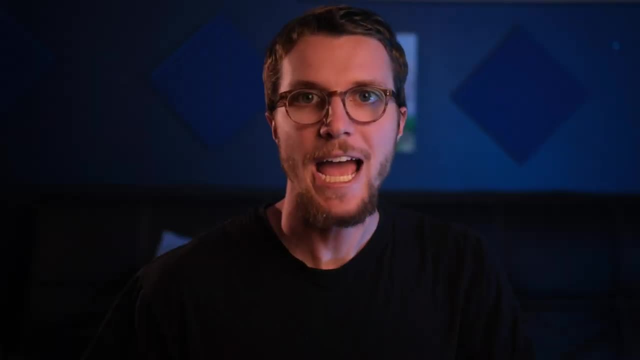 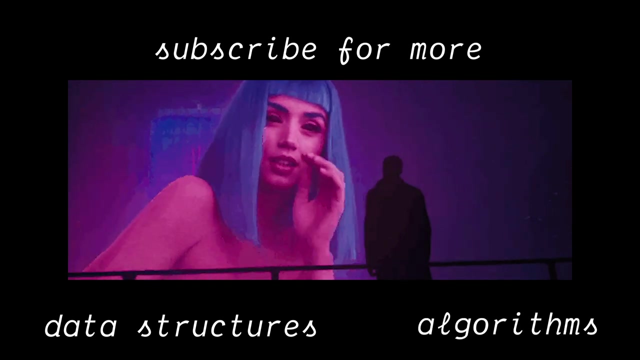 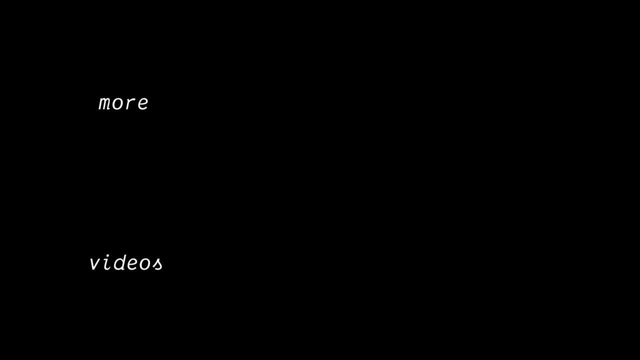 subscribe, so i'll see you in the next one. bye, bye. more people can see the video anyway, i will catch you guys soon. you want to see more videos like this? please subscribe to the channel and turn on the bell so you don't miss any of the latest videos. and don't forget to like and subscribe to the channel. bye you.